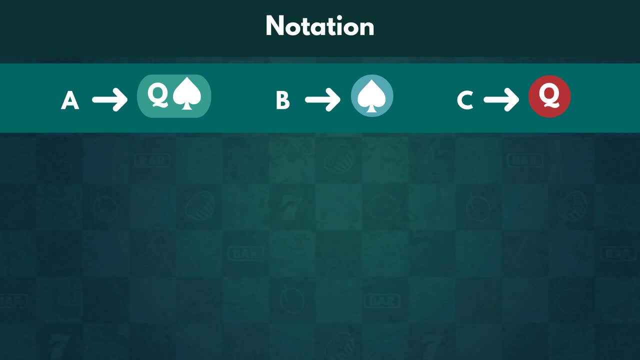 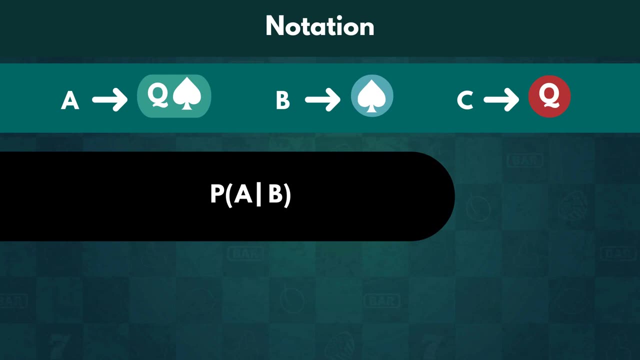 Let's formalize these observations with a formula. By definition, the conditional probability of an event A given an event B equals the probability of the intersection of A and B Over the probability of event B occurring. This holds true if the probability of event B 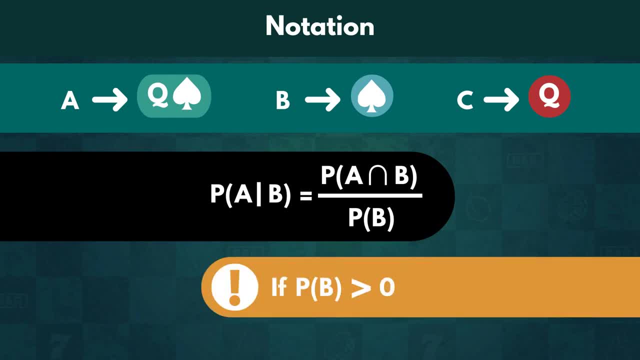 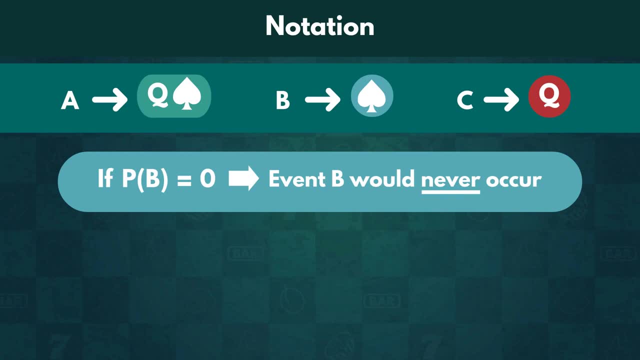 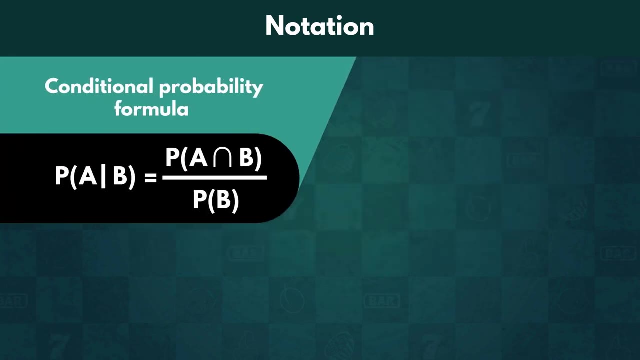 is greater than zero only, And logically so, If P of B is equal to zero, then event B would never occur. Thus A given B would not be interpretable. Now let's look at the conditional probability formula more closely. If we compare it to the favorable over all formula, we can see many. 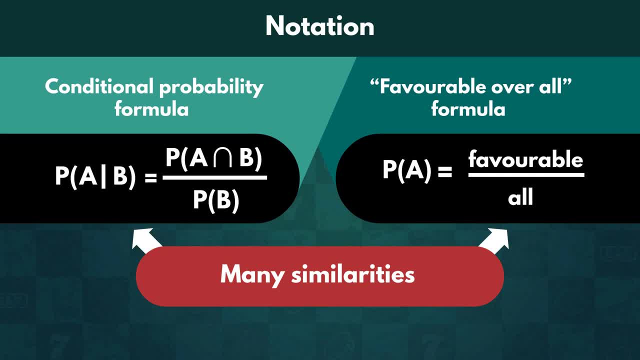 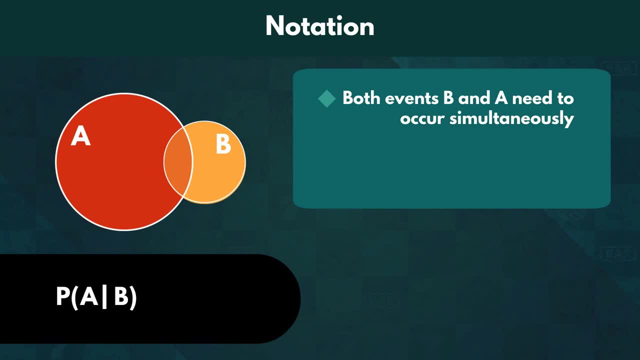 similarities. To satisfy the conditional probability, we need both events B and A to occur simultaneously. This suggests that the intersection of A and B would consist of all favorable outcomes for this probability. Secondly, the conditional probability requires that event B occurs, so the sample space would simply be all outcomes where event B is satisfied. 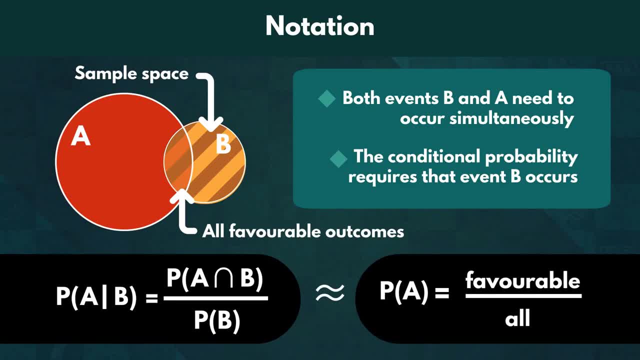 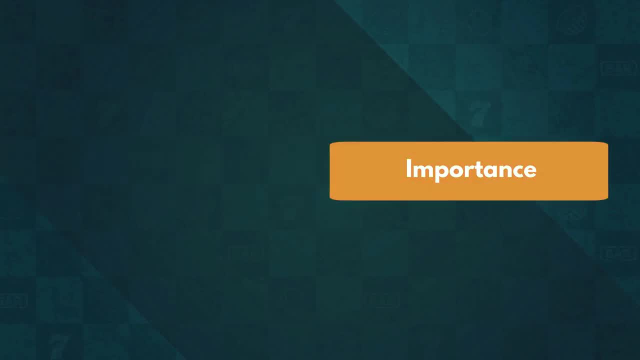 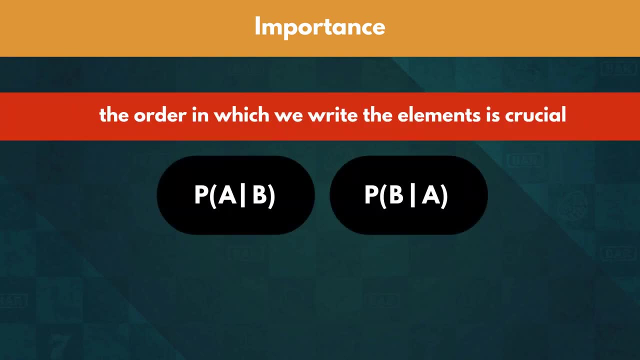 Everything fits into place now, doesn't it Great. Once we know the intuition behind the formula, we can focus on the importance of conditional probability. Firstly, try to remember that the order in which we write the elements for the conditional probability is crucial. P given B is definitely not the same as P given A. 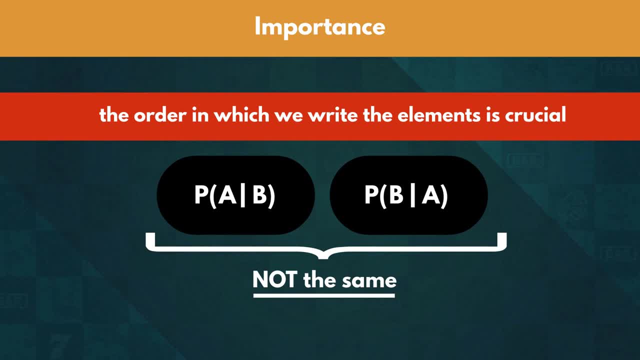 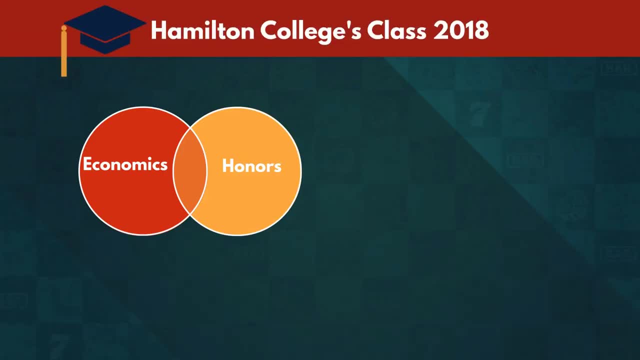 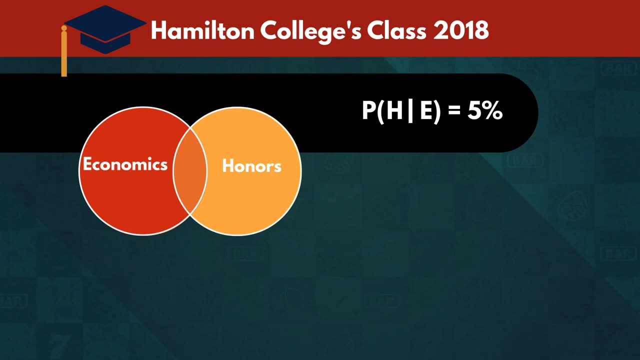 even if the numeric values are equal. For instance, let's explore the characteristics of Hamilton College's class of 2018.. How many students did we have in 2018?? Five percent of the students who got a degree in economics graduated with honors. At the same time, five percent of all students who graduated with 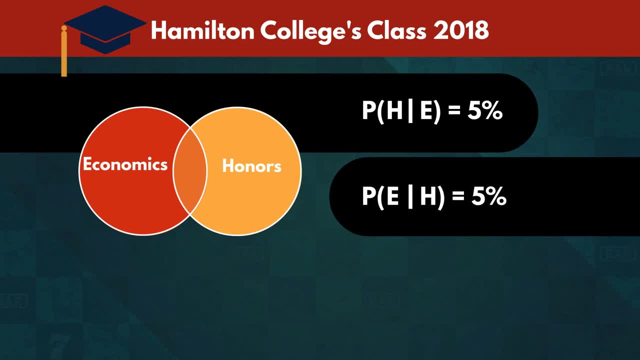 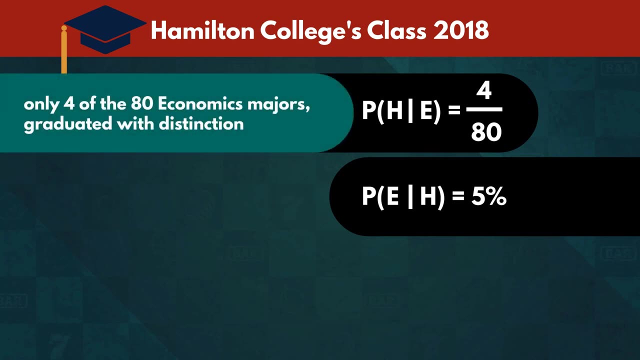 honors completed a concentration in economics. These two statements might have the same conditional probability, but they hold completely different meanings. In particular, the first one suggests that only four of the 80 economics majors graduated with distinction. The second one suggests that 4 out of the 80 students who graduated with high grades 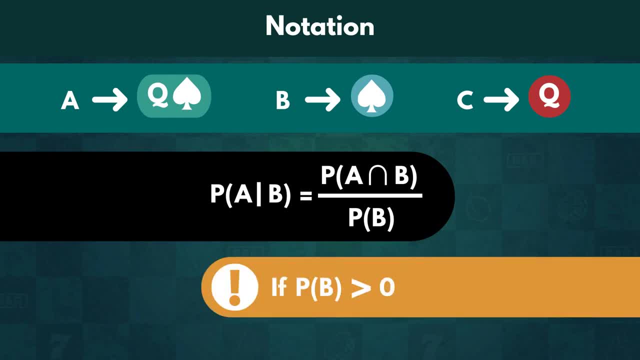 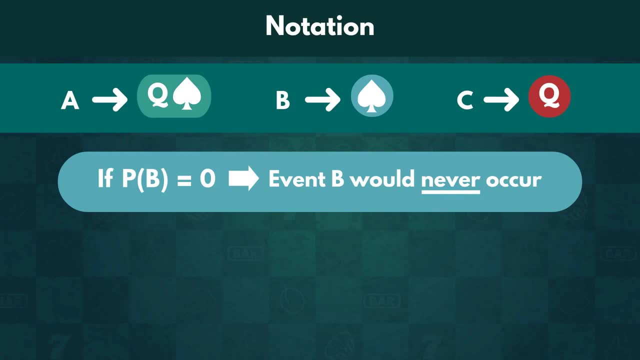 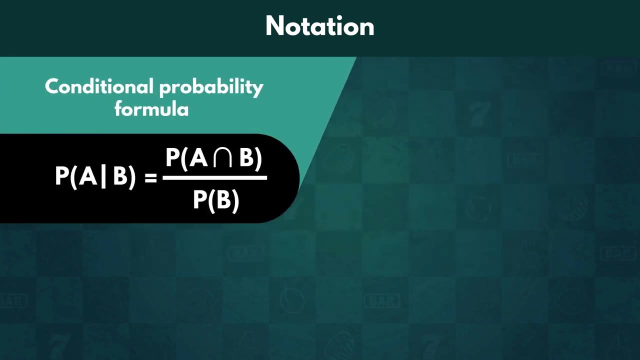 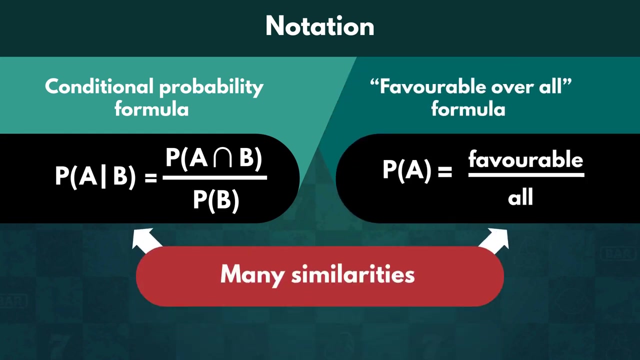 B is greater than 0 only, And logically so, if P is equal to 0, then event B would never occur. Thus A given B would not be interpretable. Now let's look at the conditional probability formula. If we compare it to the favorable over all formula, we can see many similarities To. 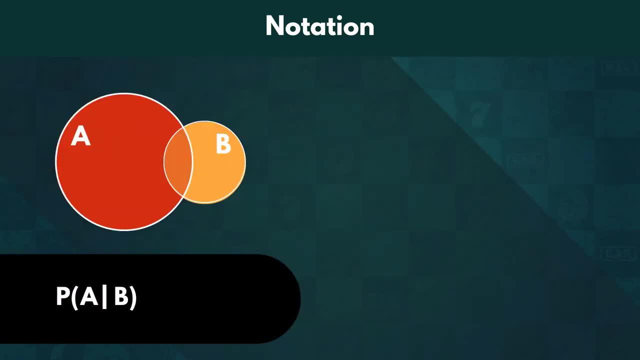 satisfy the conditional probability, we need both events B and A to occur simultaneously. This suggests that the intersection of A and B would consist of all favorable outcomes for this probability. Secondly, the conditional probability requires that event B occurs, so the sample space would 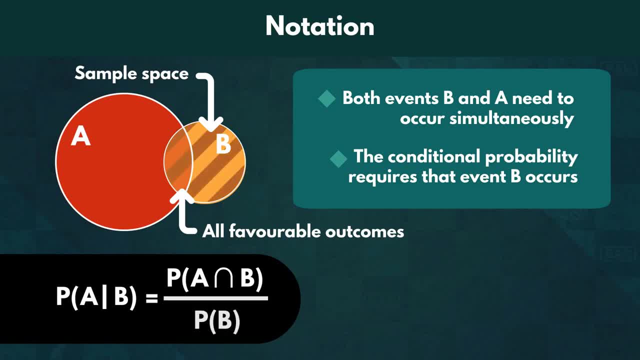 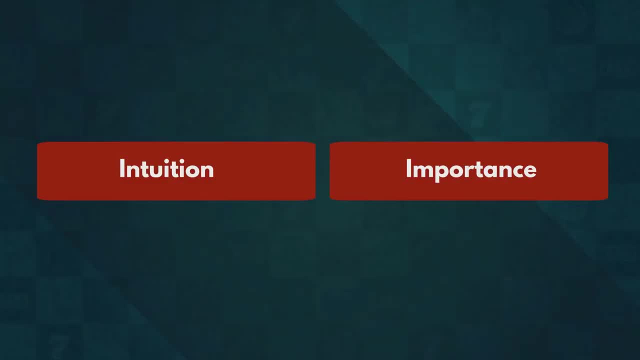 simply be all A and B. Now, if we compare it with the order of events B and A, we can see all outcomes. where event B is satisfied, Everything fits into place. now, doesn't it Great? Once we know the intuition behind the formula, we can focus on the importance. 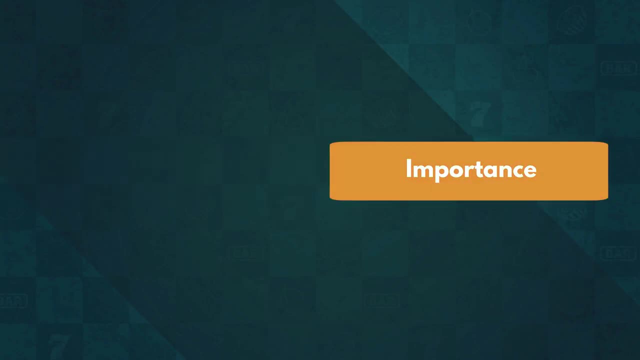 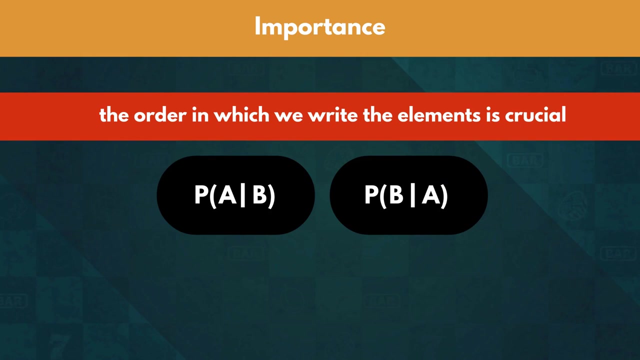 of conditional probability. Firstly, try to remember that the order in which we write the elements for the conditional probability is crucial. P given B is definitely not the same as P given A, even if the numeric values are equal. For example, if A is equal to B and B equals A, then P of B is equal to B. If P of A is equal to B, then P of B is equal to A, even if the numeric values are equal. If P of B is equal to B, then P of B is equal to A, even if the numeric values are equal. 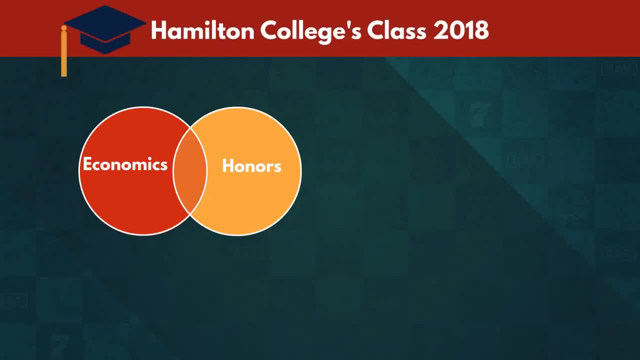 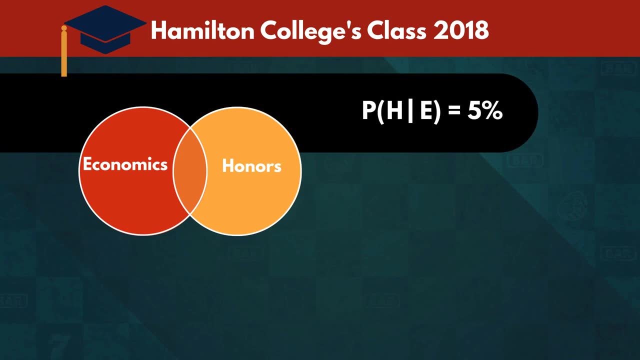 For example, if the number of MC is equal to B, then C is equal to C instance. let's explore the characteristics of Hamilton College's class of 2018.. 5% of the students who got a degree in economics graduated with honors. At the same time, 5%. 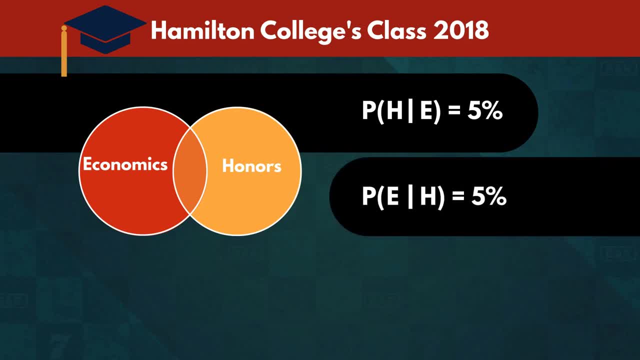 of all, students who graduated with honors completed a concentration in economics. These two statements might have the same conditional probability, but they hold completely different meanings. In particular, the first one suggests that only four of the 80 economics majors graduated with distinction. The second one suggests that four out of the 80 students 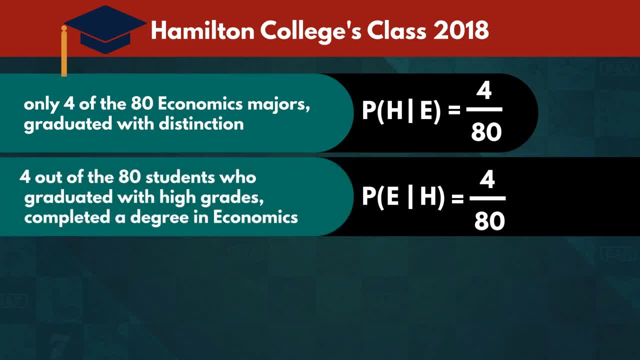 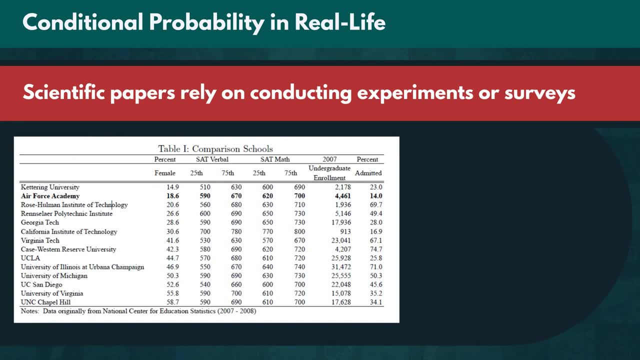 who graduated with high grades, completed a degree in economics. Many scientific papers rely on conducting experiments or surveys. They often provide summarized statistics we use to analyze and interpret how certain factors affect one another. An example would illustrate this better. Imagine you conducted a survey where 100 men and women of all ages 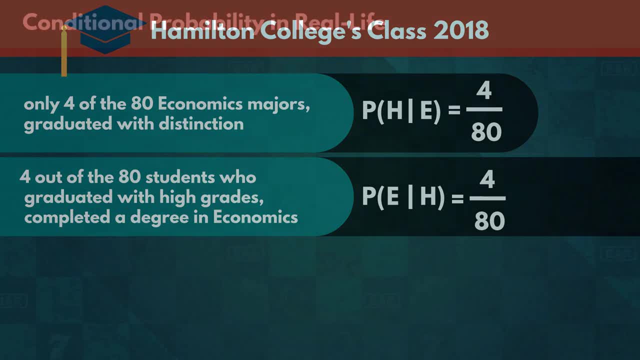 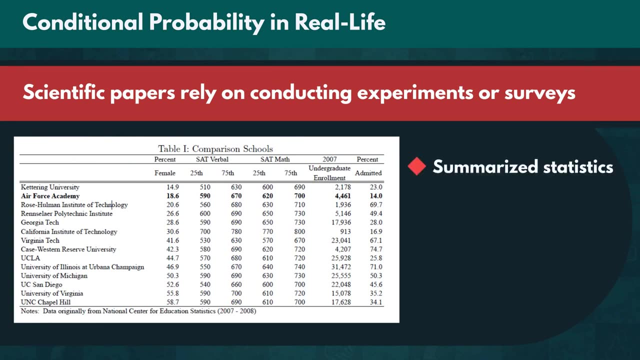 completed a degree in economics. Many scientific papers rely on conducting experiments or surveys. They often provide summarized statistics we use to analyze and interpret how certain factors affect one another. An example would illustrate this better. Imagine you conducted a survey where 100 men and women of all ages 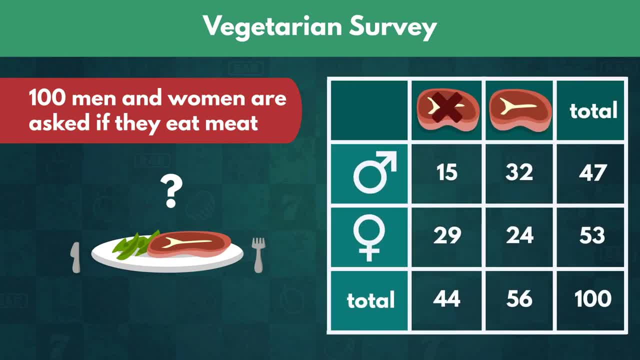 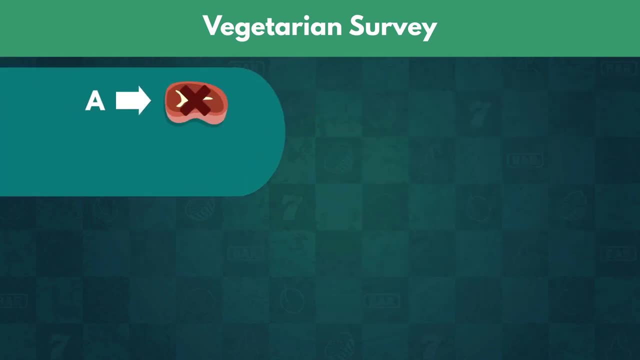 were asked if they eat meat. The results are summarized in the table. on the screen We see 15 of the 47 women that participated are vegetarian, as are 29 out of the 53 men. Now, if A represents being vegetarian and B represents being a woman, 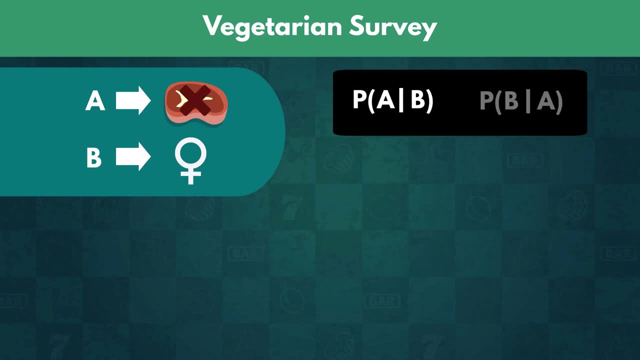 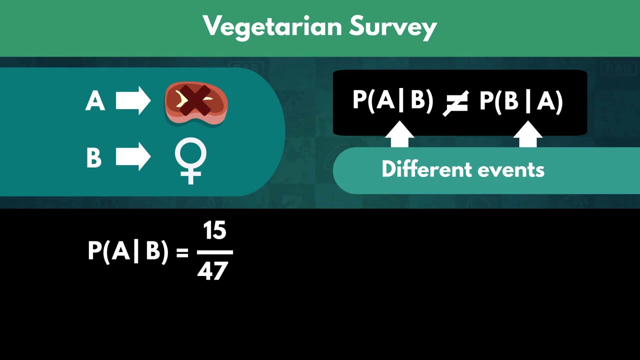 then, P of A given B and P of A given A express different events. The former equals 15 over 47 and represents the number of women who participated in the survey. P of A represents the likelihood of a woman being vegetarian, while the latter equals 15 over 44. 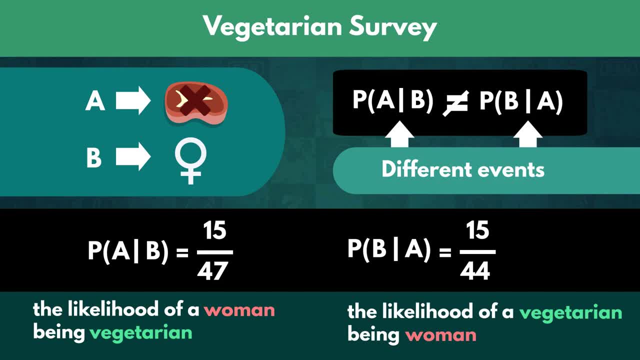 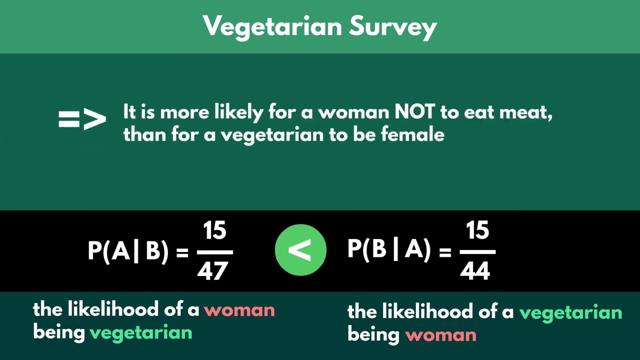 and expresses the likelihood of a vegetarian being a woman. Since 15 over 44 is greater than 15 over 47, it is more likely for a woman not to eat meat than for a vegetarian to be female. That's quite interesting and shows you that, in probability theory, 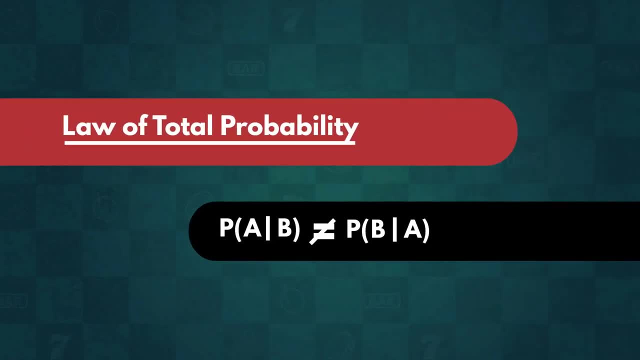 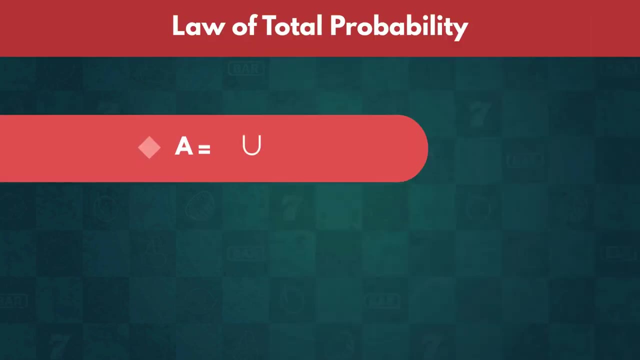 things are never straightforward. Now that you understand the theory of probability and that you understand the distinctions between the different conditional probabilities of two events, we can introduce an important concept: the law of total probability. Okay, Imagine: A is the union of some finitely many events. 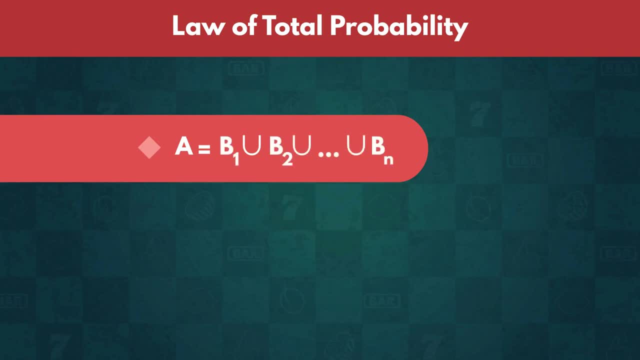 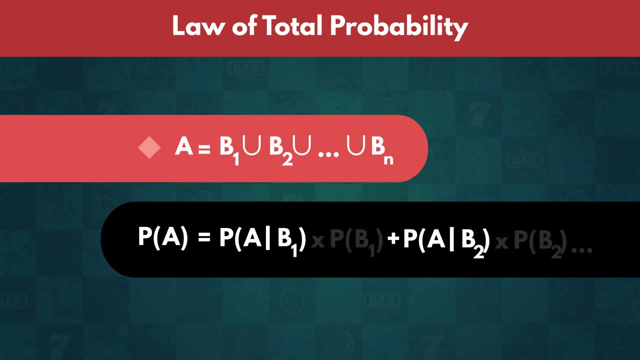 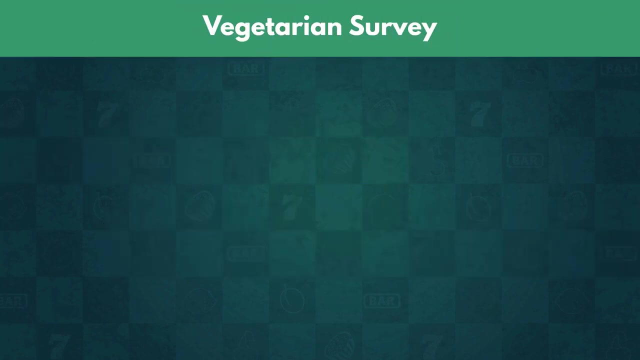 B1,, B2, and so on. This law dictates that the probability of A is the sum of all the conditional probabilities of A given sum B multiplied by the probability of the associated B. To clear any confusion, let us go back to the survey example. 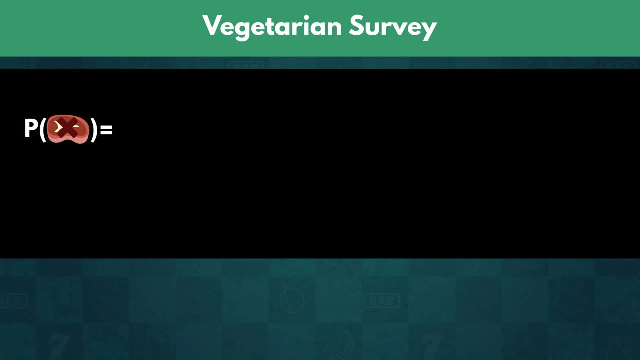 The probability of being vegetarian equals the sum of the probability of being a vegetarian, given the person is male, times the probability of being male, and the probability of being a vegetarian, given the person is female, multiplied by the probability of being female, If we plug in values from the table. 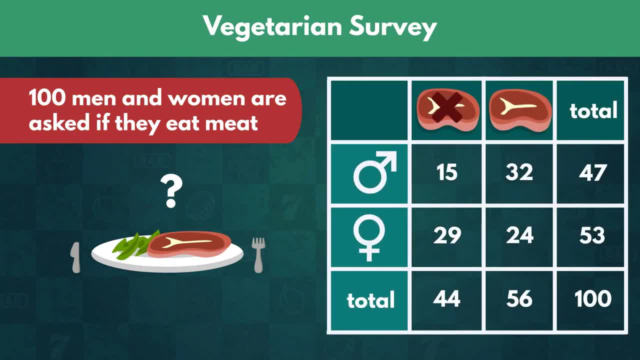 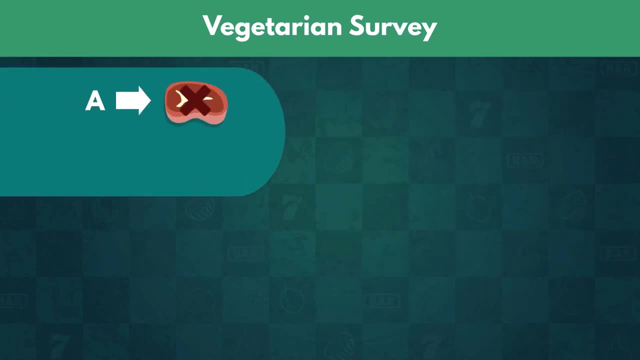 were asked if they eat meat. The results are summarized in the table. on the screen We see 15 of the 47 women that participated are vegetarian, as are 29 out of the 53 men. Now, if A represents being vegetarian and B represents being a woman, then P of A given B and P of 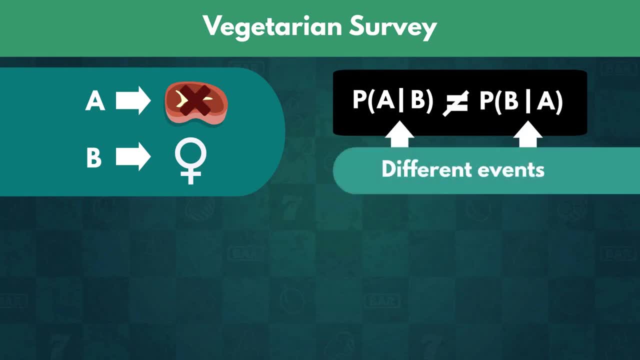 A given B are equal. If A represents being a woman, then P of A given B and P of A. given A represents being a woman, then P of A given B and P of A represents being a woman, then P of A given A express different events. The former equals 15 over 47 and represents 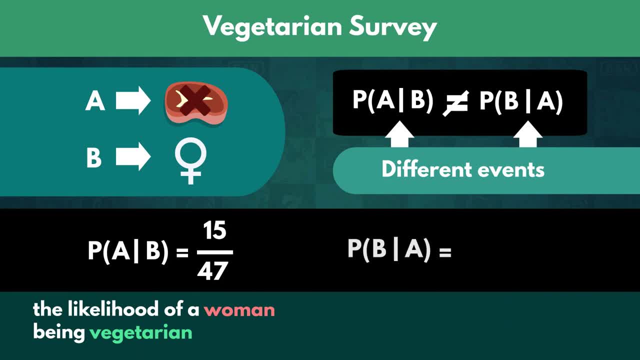 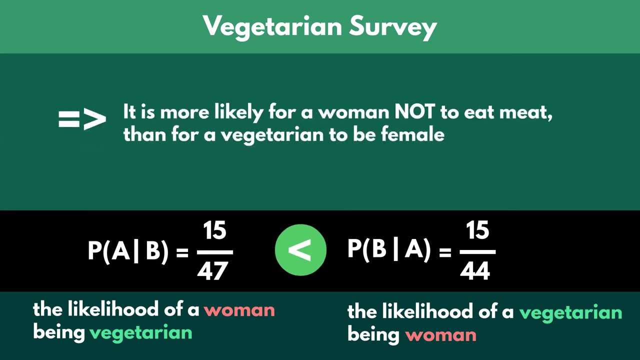 the likelihood of a woman being vegetarian, while the latter equals 15 over 44 and expresses the likelihood of a vegetarian being a woman, Since 15 over 44 is greater than 15 over 47, it is more likely for a woman not to eat meat than for a vegetarian to be female. That's. 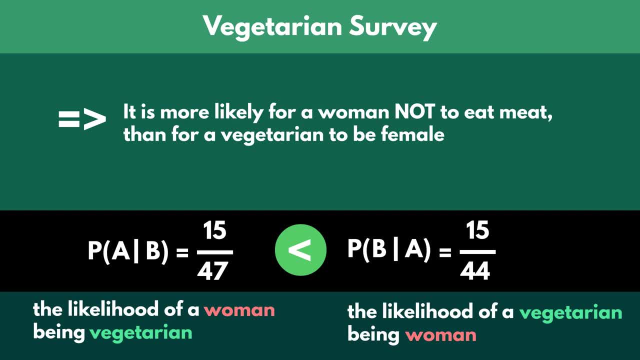 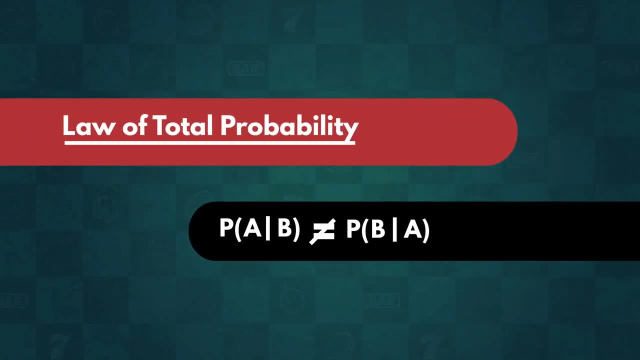 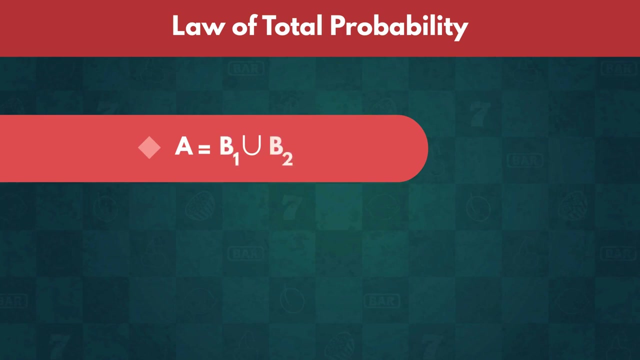 quite interesting and shows you that in probability theory things are never straightforward. Now that you understand the distinctions between the different conditional probabilities of two events, we can introduce an important concept: the law of total probability. OK, Imagine A is the union of some events: B1,, B2, and so on. This law dictates that the probability of A is the sum of 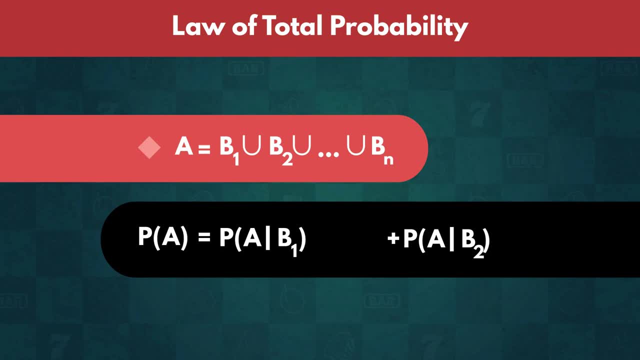 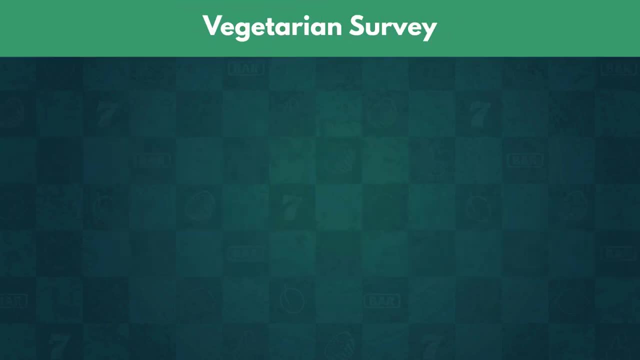 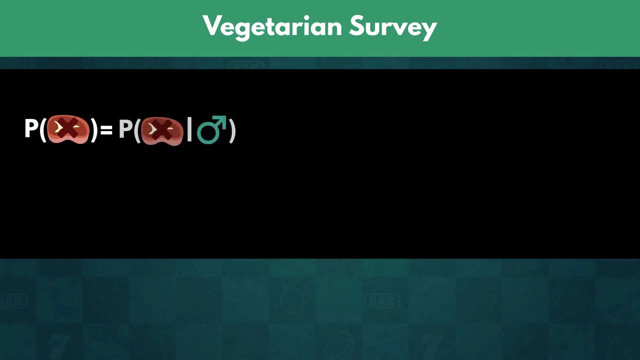 all the conditional probabilities of A given sum, B, multiplied by the probability of the associated B. To clear any confusion, let us go back to the survey example. The probability of being vegetarian equals the sum of the probability of being a vegetarian, given the person is male, times the probability of being male and the probability of being a vegetarian. 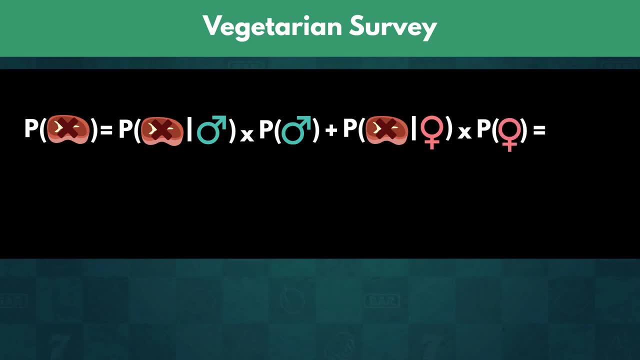 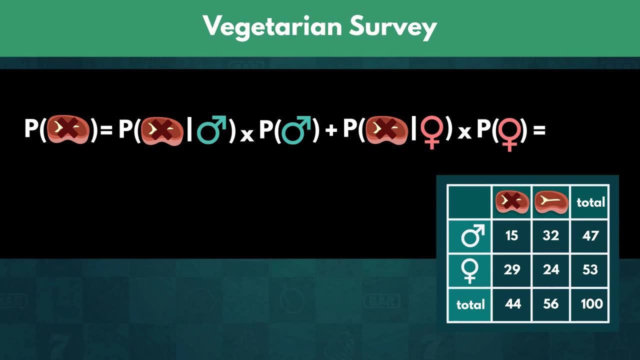 given the person is female, multiplied by the probability of being female, If we plug in values from the table, we get the probability of being vegetarian equals twenty nine over fifty three times fifty three over one hundred, plus fifteen over forty seven times forty seven over one hundred, That's 44 over 100 or .44.. Therefore, according to, 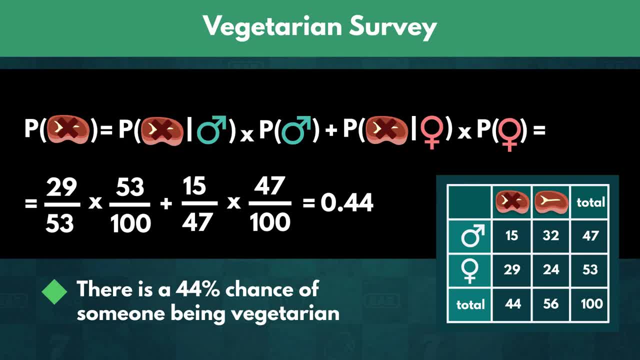 the survey, there is a 44% chance of someone being vegetarian. We can refer back to the example to say that the possibility of being a vegetarian is greater than the probability of being a female. The probability of being a vegetarian is 0.44.. Therefore, according to the survey, there is a 44% chance of someone being vegetarian. 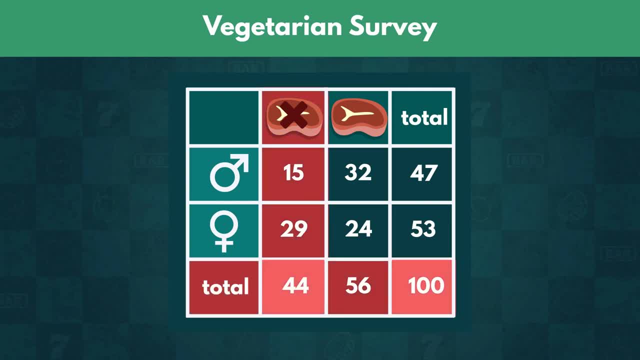 table and confirm the probability of being vegetarian is indeed 0.44.. So our answer checks out. 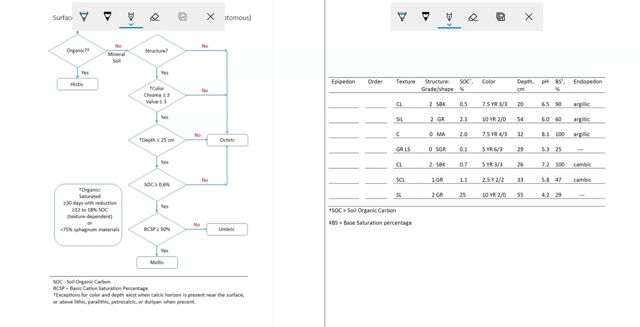 One part of the study guide has descriptions of the properties of individual horizons. In this case, we're talking about surface horizons or epipedons, And so we have the texture, we have the structure, we have the color, and then we have some additional information that we may need for this. 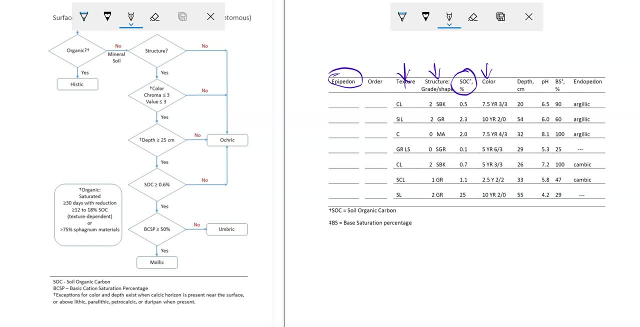 One of those is the soil organic carbon. You saw the cross there. You always look for footnotes to figure out what that is about. And then the base saturation may become important to us and we see. how do we know? that's what we're looking at. 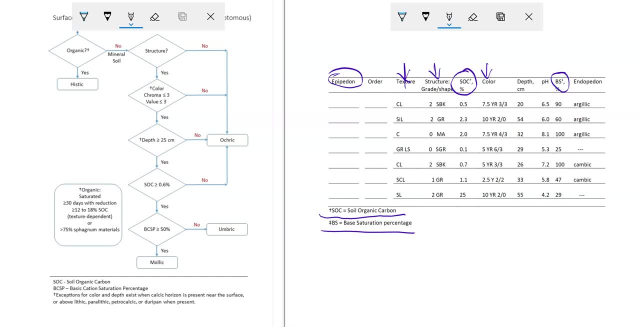 Well, again, we look for the footnote symbol and we look to find what is that? So we have these definitions. We've got, then, a description of physical and chemical properties of an individual surface horizon. We then switch to use the dichotomous key that's available for us. 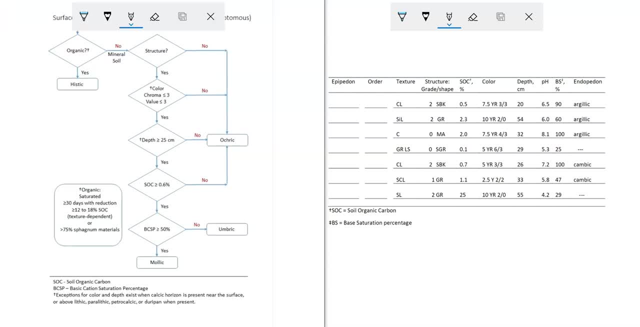 And so we look here and we have a surface or epipedon key And it's a dichotomous key, meaning it's a series of yes or no questions. So we're going to look at the properties of the soil of that horizon. 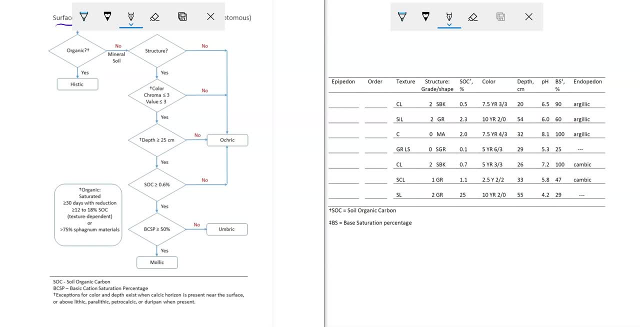 and we're going to use that apply this Series of questions we have over here, Dichotomous key works. you have a rhombus that's a question And then you have a series. you either go one direction or other, depending on your answer.